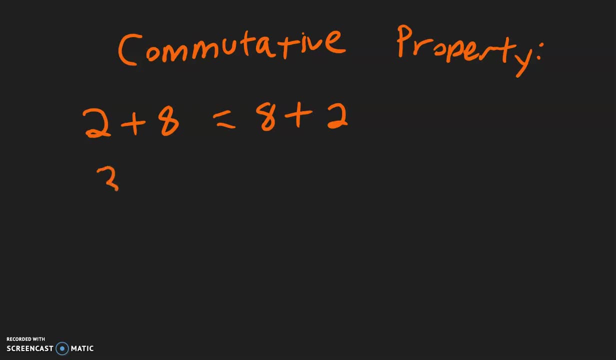 commutative property with multiplying. For example, 3 times 7 is 21.. So is 7 times 3.. So this is also true. Here's another example: Negative 2 plus 9 is the same as 9 minus 2.. And this one is not very obvious at first, but when you look at this, 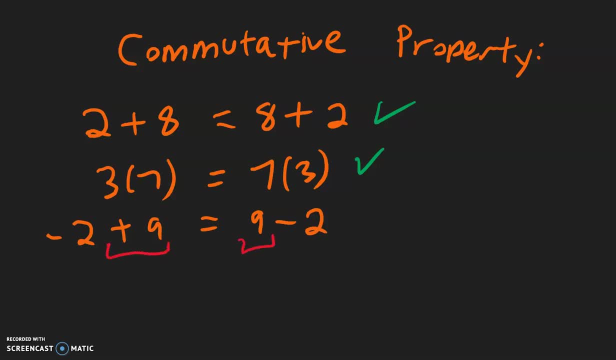 you see how the 9 was positive, the 2 was negative And if you calculate both sides, negative- 2 plus 9 is 7, and 9 minus 2 is also 7.. So, according to the commutative property, 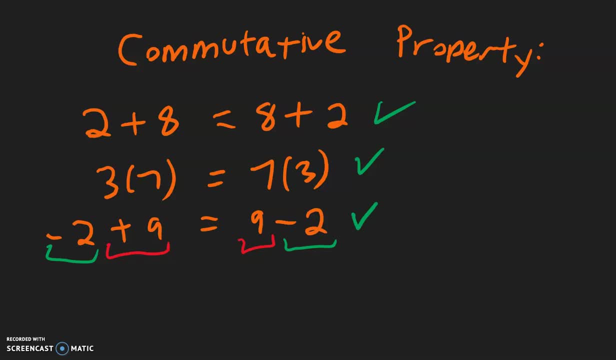 this is also true. And now for the final example. The final example here is when it is not true. You have 2, 2 minus 9 and 9 minus 2.. And these are not equal because, see, the 2 was positive over here. 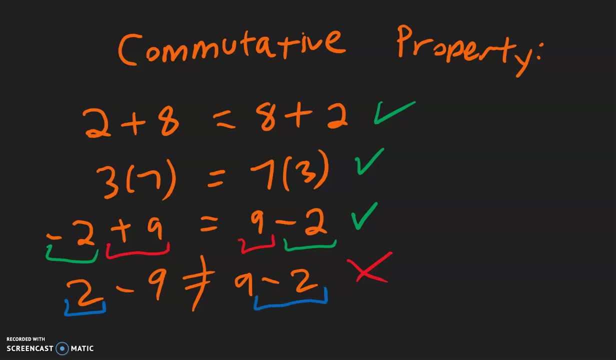 but it was negative over here, So that's not going to be the same. And for the 9,. you also see the signs are different on both sides. So here's how the commutated property is useful in algebra. Let's say you have an expression and then your value is 2 minus 5x. but 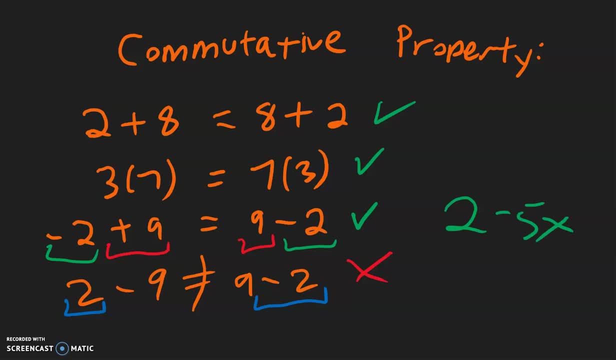 you want to get the term with the x in front, so you can just flip this as negative: 5x plus 2.. And this would be exactly the same thing, because the 5x was negative and stayed in negative and the 2 was positive and it stayed. 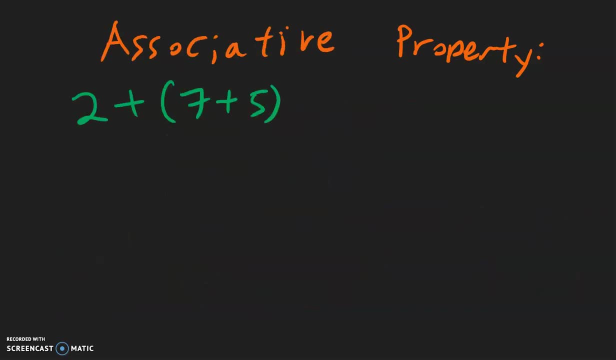 positive. Now we will talk about the associated property. In this example we have 7 plus 5 inside the parentheses. So the parentheses tells you that we're going to do that first. So 7 plus 5 is going to be 12, and plus 2, that's going to be 14.. But what associated property tells you is: 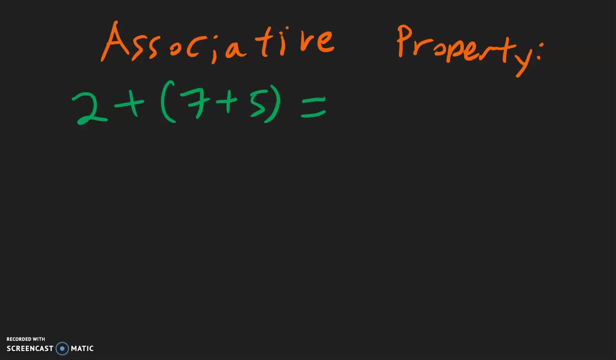 that you can change the grouping So you can think of grouping as like associating. So I'm going to change the grouping to have the 2 plus 7 come first and then we will add 5 later on. So 2 plus. 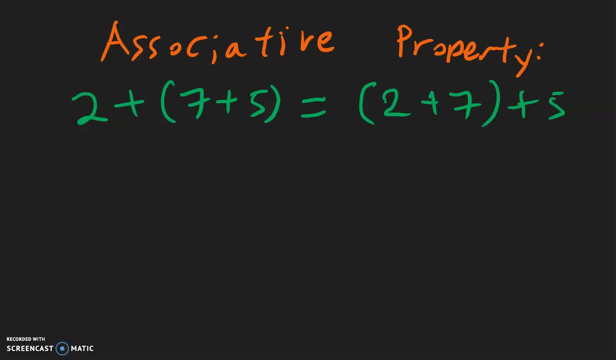 7 is going to be 9, plus 5,, it is still 14.. Let's do an example with multiplication. So we can do 5 times 2 multiplied with 3. So 5 times 2 is 10.. 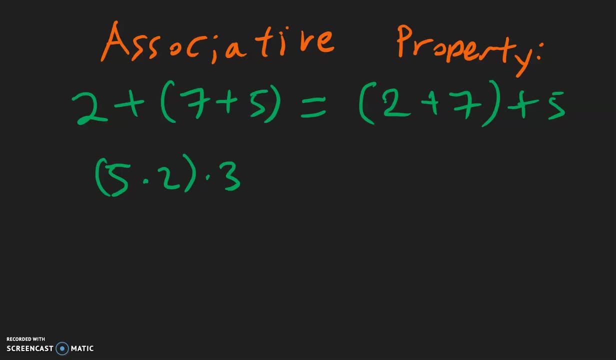 And we did that first because that's inside the parentheses, And 10 times 3 is 30.. Now let's see what happens if we change the grouping symbol. So 5 is going to be outside of the parentheses now, but we have 2 times 3 inside the parentheses, So we will do the 2 times 3 first, which is 6,. 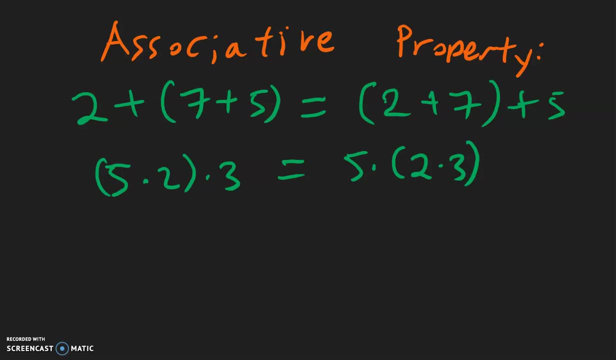 and then multiply that with the 5 on the outside, which is still 30. And so whenever you see the grouping, the parentheses symbol change. that's the associated property. You are changing the association, you're changing the group. And the last property we will be talking about in this video is the distributed property. 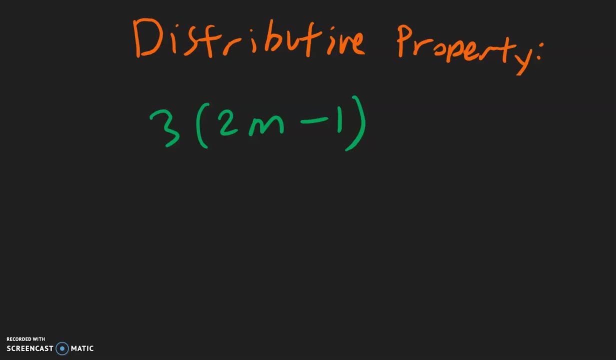 So this one is the one that most people are very familiar with. When you see this, you know, to multiply 3 times 2, m is going to be 6m, and 3 times negative 1 will be negative 3.. But why do we even need the distributed property? Well, here's why I am going to 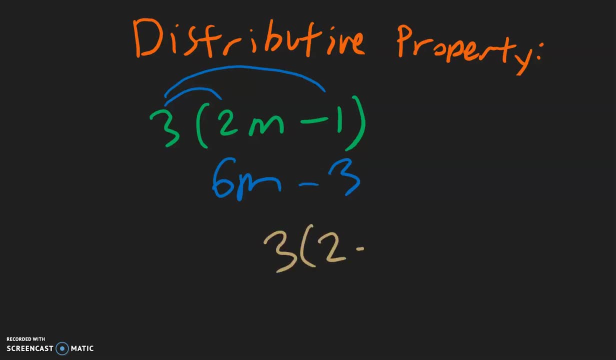 write an example that is really similar to this, except that we don't have m, In this case parentheses- tells us to do that first. So 2 minus 1 is going to be 1, then 3 times 1 is going to be 3.. And we can do that, no problem. But going back to the 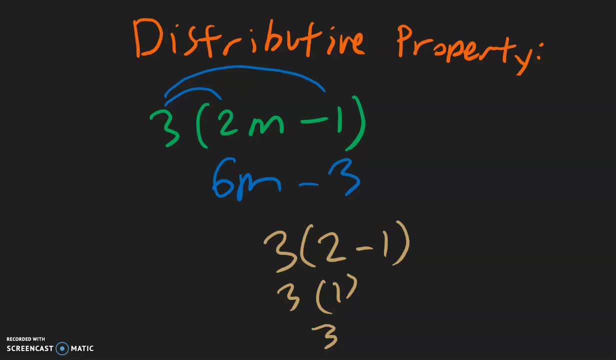 expression in green. we have 2m minus 1, and they are not like terms, So we cannot just combine it together, even though parentheses is telling us do that first, But we can't, and so we can't do that, So we can't do that, So we can't do that, But we can't do that. 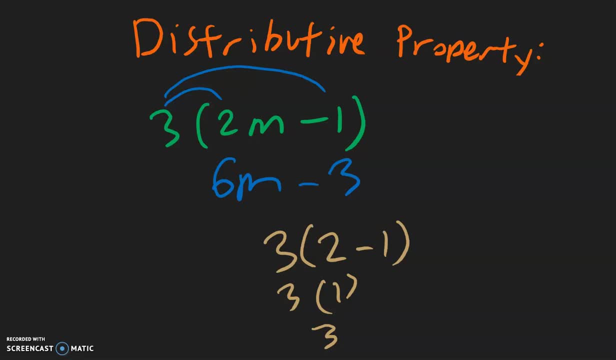 distributed property is. I could go around that says okay, well, I can't combine the 2m and the negative 1, but I can multiply it by 3 first, so so we can distribute that. so here we have three statements, and for each one we are going: 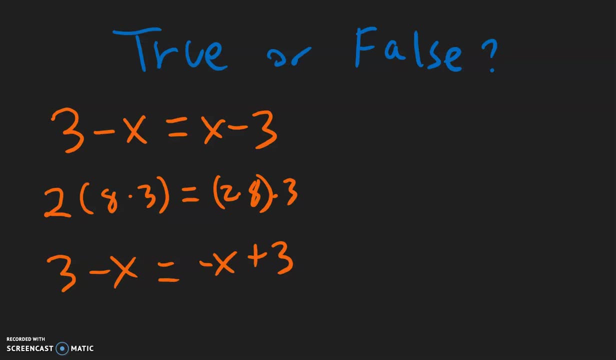 to see if they are true or false, and if they're true, we'll write down the property that makes it true. so the first one is going to be false. so this looks like this is the the commutative property. but here's a problem, see this. 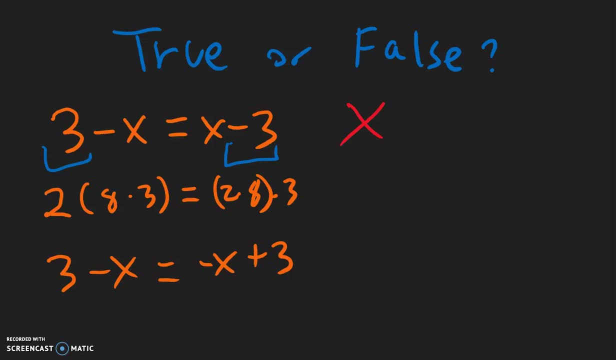 3 was positive and now here is negative, so they're not gonna be the same. the second one is true, and it is true because of the associated property. we see the grouping change. right, it used to be grouped with eight times three first and else group with the two times eight first. so this is true because of the 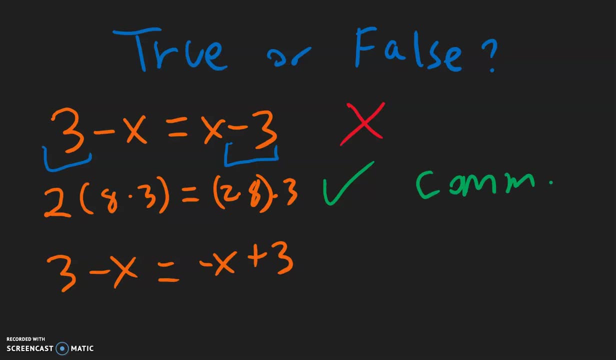 commutative property. and the last one is true. this is the oh. sorry, I made a mistake on the last one. this, this is the associative property. right, we're changing the association associative, okay. and the last one is the commutative property. and this one is true because, you see, the three was positive and it stays positive, but the X was negative. 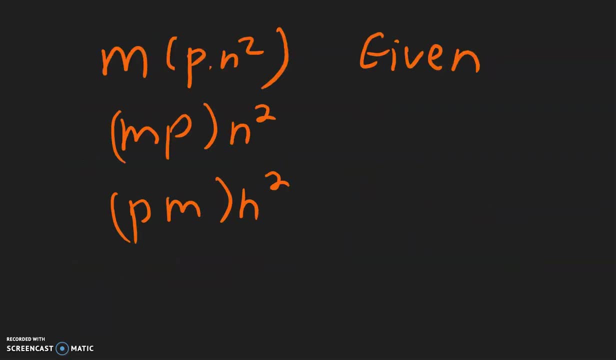 and I also stayed negative for this example. on the left side we have a series of steps and on the right side we're going to give the reason why we can do this step. okay, so what happened between the first and second steps? over here, the grouping symbol change, and so 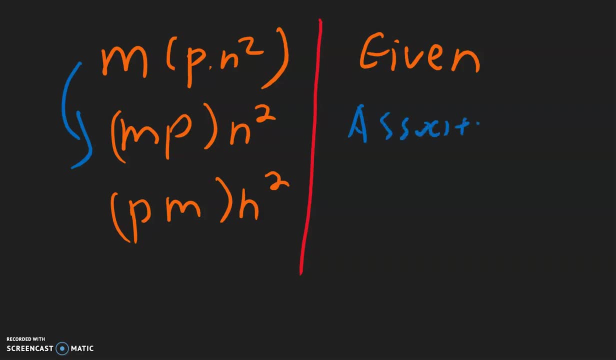 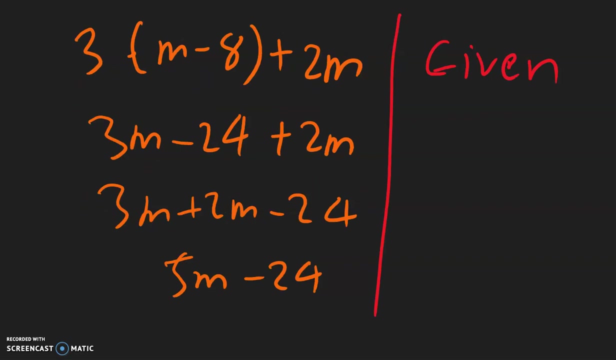 we know that's going to be the associative property. and then, over here, what changed was that the m in the P, which is being multiplied, is being reversed, and so reversing that's the commutative property. and for our last example, we will write down the properties for each step. so what happened between the first line and the? 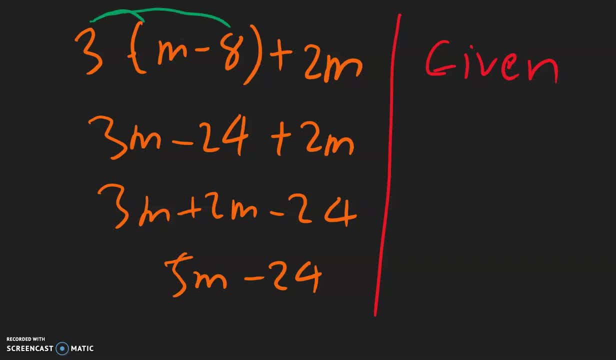 second line. well, we were multiplying, so that's called distributive property. and what happened between the second line and the third line is that the negative 24 and the positive 2m, they switched places. and so after they switch places, you see how the negative 24 still stay negative 24 and the positive 2m is still